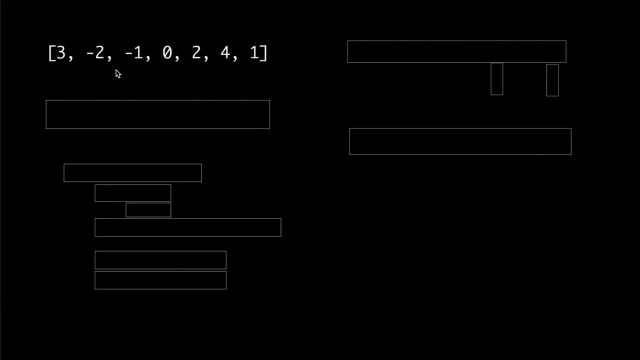 So suppose you're given an array of integers, for example this one, and your task is to sort it in the ascending order, just like that. And one approach you can use for this is quicksort. Quicksort implements a recursive function, which we're going to call qs, that takes three arguments. 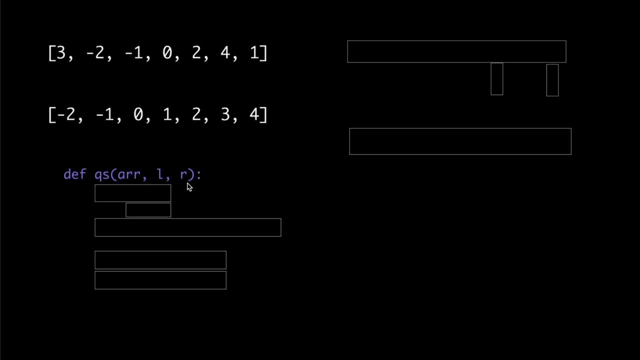 The given array, l and r. l and r will be two integers that are going to represent the indexes that will show the section of the array that we want to sort. So, for example, if you're given this array and if l happens to be 5,, 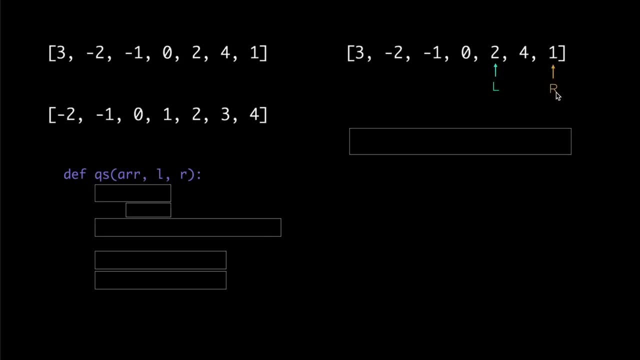 the index of this element right here and r happens to be 6, the index of this element right here. then, after running this function with these particular arguments, this array will be like this. So the section of the array that's between l and r will be sorted just like that. 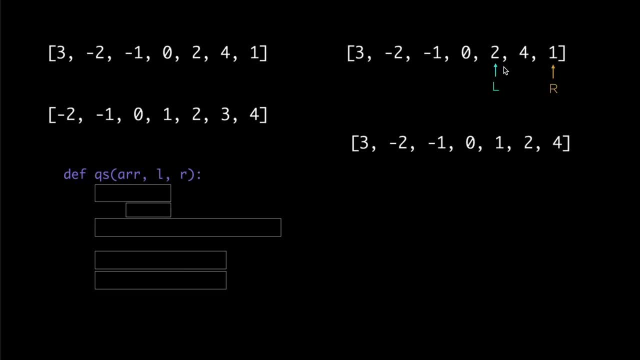 So if you want to sort the entire array using qs, you just need to give the same array, with l being the index of this element right here and r being the index of this element right here. So if you want to sort the entire array using qs, you just need to give the same array. 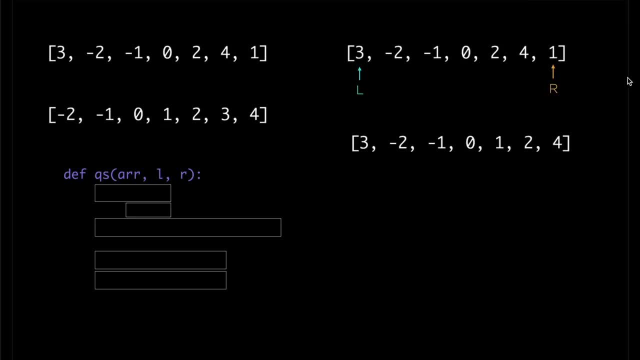 with l being 0, the index of the first element and r being 6, in this particular case, the index of the last element, And to implement this recursive function, qs, we'll first take care of the base case, That's, when l is greater than or equal to r. 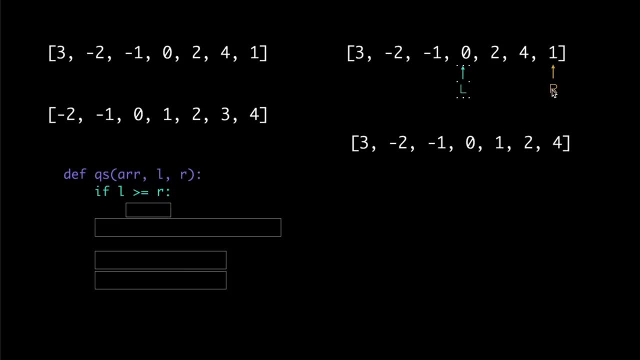 If l is equal to r, if they're pointing to the same element, for example this one, then that will mean that the section of the array that we want to sort has only one element. That's already sorted, so there's nothing to do. 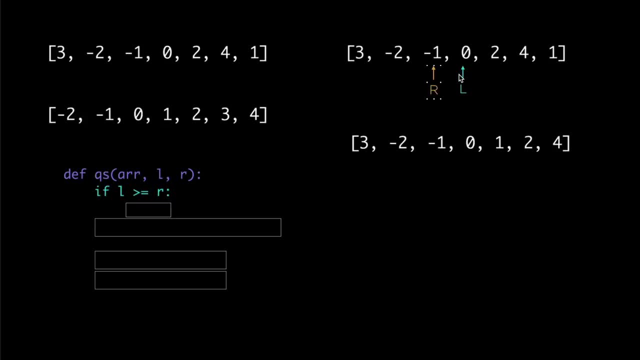 And if l is greater than r, it's sort of the same thing. The section of the array that we want to sort has no elements, so there's nothing to do, and that means we can just return from this function. Okay, so that's the base case, but what about the recursive case? 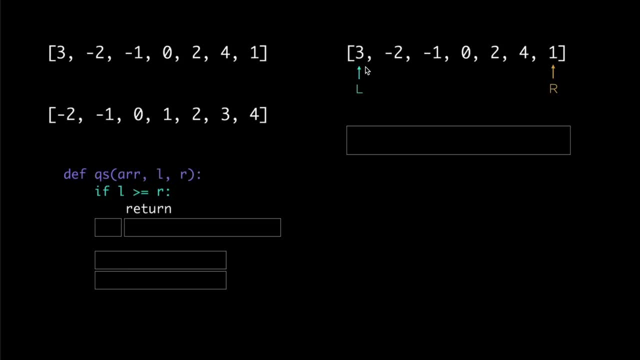 For that. let's take a look at this example here, where we're given this particular case and we're given this particular array, with l being 0 and r being 6, or the index of the last element of this array. In a recursive case, we're going to do what's called partition. 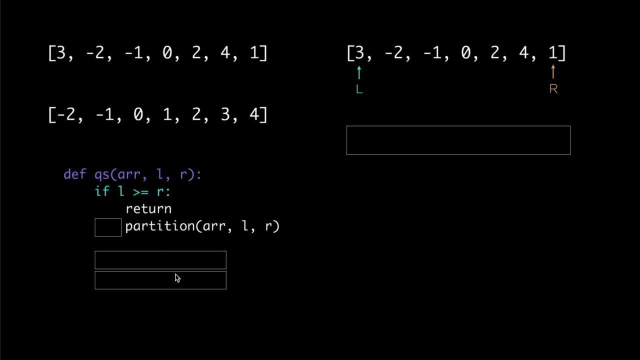 I'm going to explain what it is in a second, but for that we're going to use this function called partition. that takes three arguments, just like qs. It's going to take r, l and r, And this is going to do what's called partition for the array. 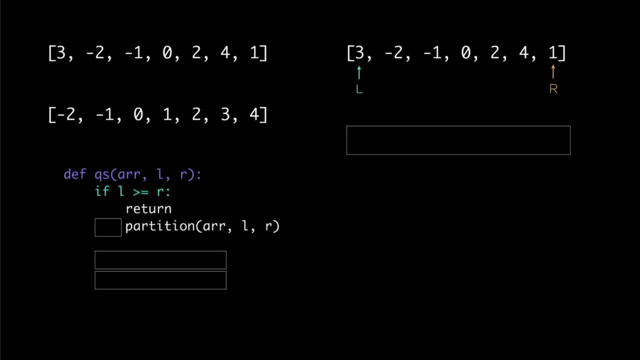 for the section of the array and the section between l and r. So let me explain what it means exactly. The first step for partitioning is to pick what's called a pivot. I'm going to explain what it is in a second. 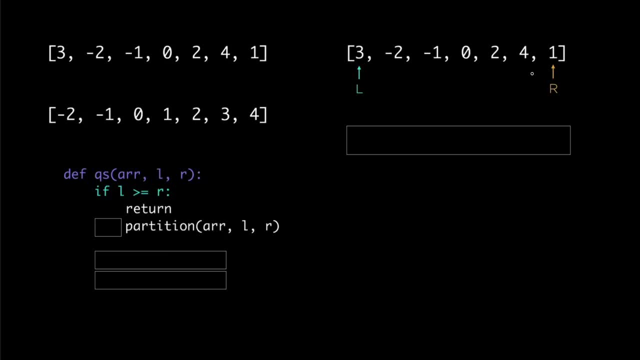 and there are different ways of choosing your pivot, but one simple approach is to pick the last element as your pivot, So that's this number right here. in this particular case, Then, the goal of this partition function is to divide this array into two groups. 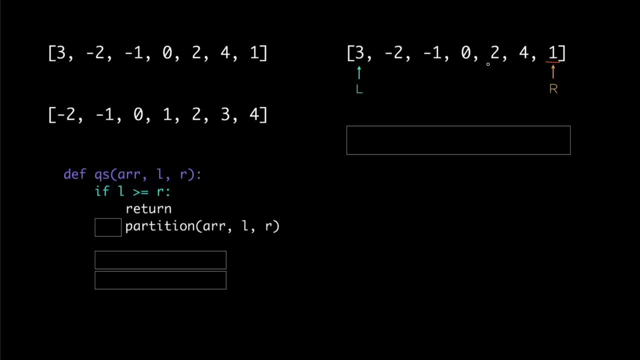 The first group is going to be all the numbers that are less than the pivot. So in this particular case, that's these three numbers minus 2, minus 1, and 0. And those numbers should come to the left of the pivot. 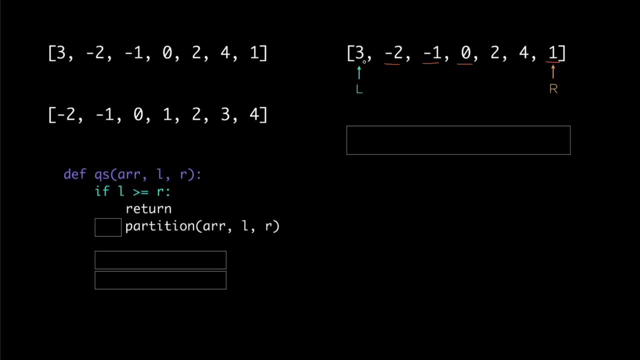 And the second group of the numbers that we're going to examine is going to be the numbers greater than the pivot. So those are these three numbers- 3, 2, and 4 in this particular case, And these three numbers should come to the right of the pivot. 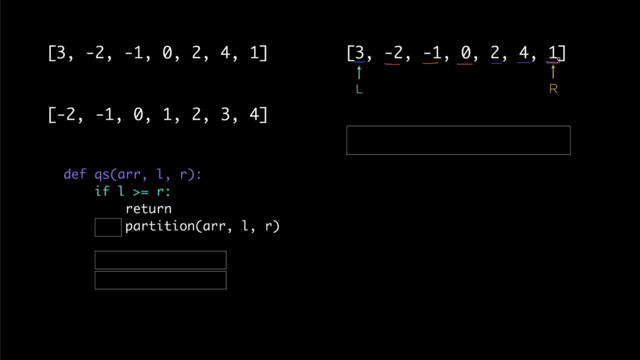 And obviously the pivot should come in between those two groups of numbers. So in this particular case, after running the partition function, the array should look like this: As you can see, after running the partition function, the pivot will come to the center of the array. 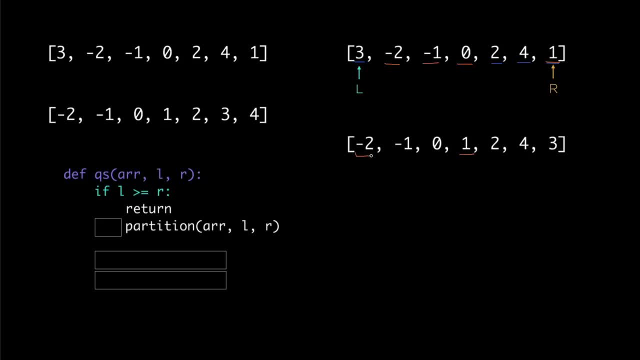 and all the numbers less than the pivot are to the left of it and all the numbers greater or equal to the pivot are to the right of it. And we don't care about the ordering of the numbers within each group. These numbers happen to be sorted. 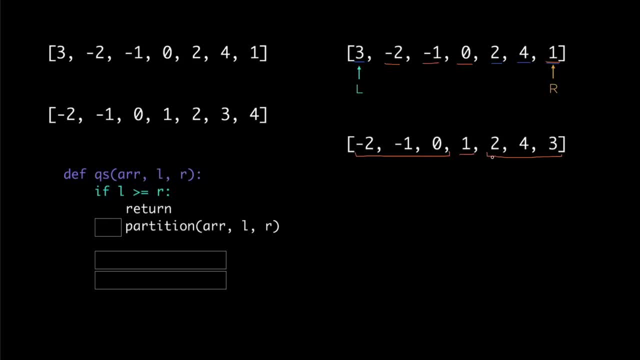 but, as you can see, these numbers in this group are not sorted Either way. another thing to note here is that we're going to write this partition function so that it's going to do that partitioning and then it's going to return the new index of the pivot. 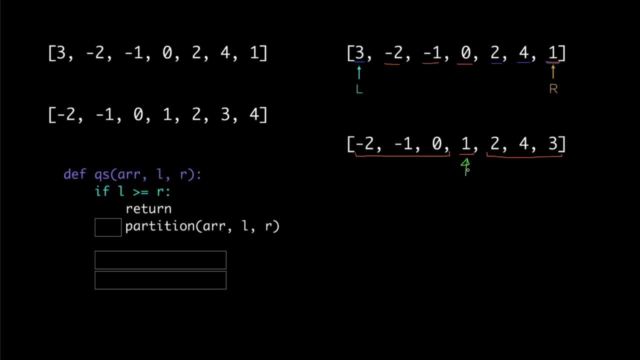 So in this particular case, that's right here, and so it's going to return 3, or the index of the pivot, And then we can store it in a new variable, which we're going to call p here, And I'm going to show you how to implement partition later. 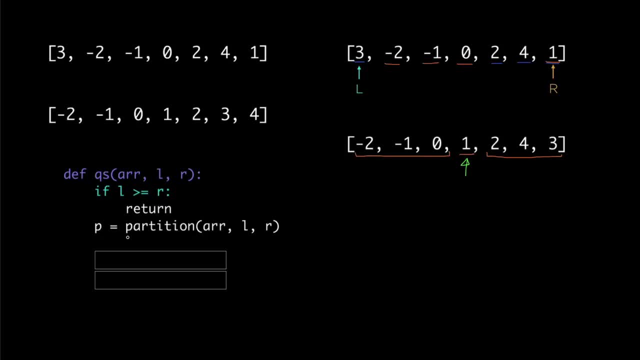 but let's just here for now, say that we already have this function. So after partitioning the given section of the array, we'll already know that the position of the pivot right here is correct. So that means that this position isn't going to change. 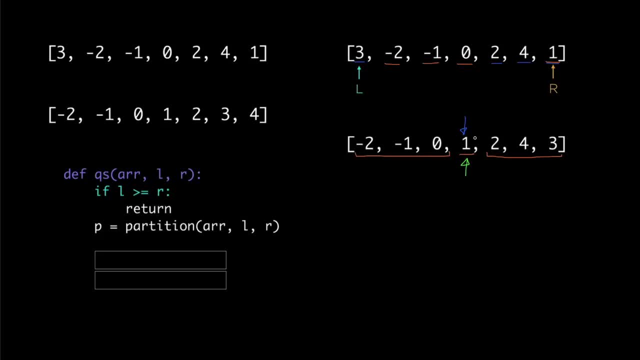 after sorting this entire array. So all we need to take care of after partitioning is this group of numbers and this group of numbers. We need to sort this section and then this section, And we can do that by calling qs on this section and then qs on this section. 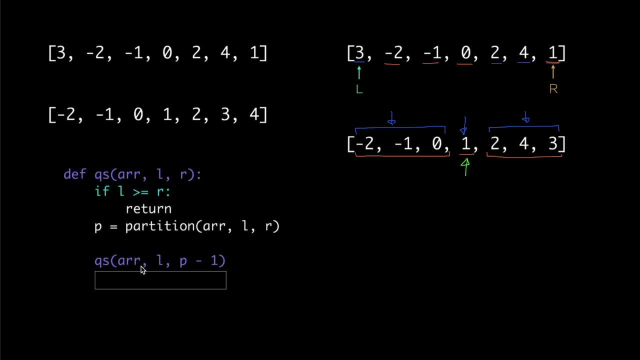 We can do that with qs of r, l and p-1.. So here we're saying we're going to sort the section of the array between l- which is right here- and p-1, which is right here, And then we're going to do the same thing for the other section. 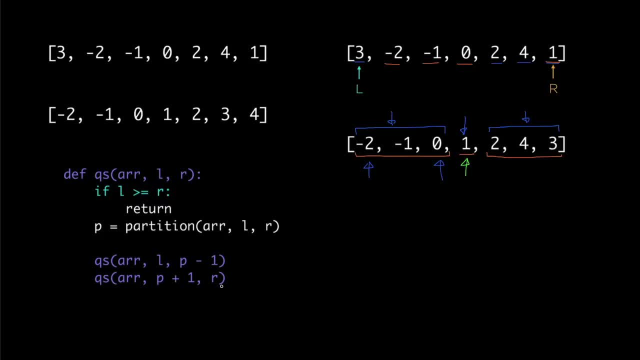 with qs of r, p-1, and r. So we're saying we're going to sort the section of the array between p-1 and r And by repeating this process recursively we'll be able to sort the entire array. Now let's take a look at how partition might be. 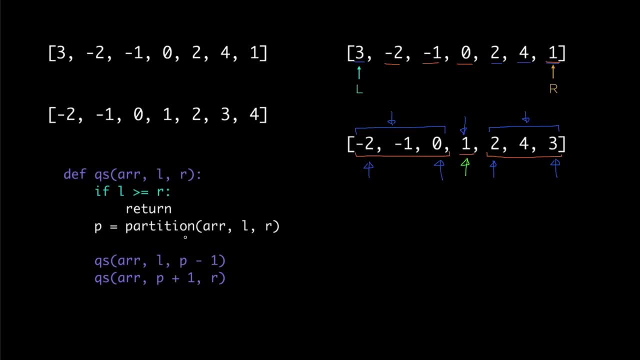 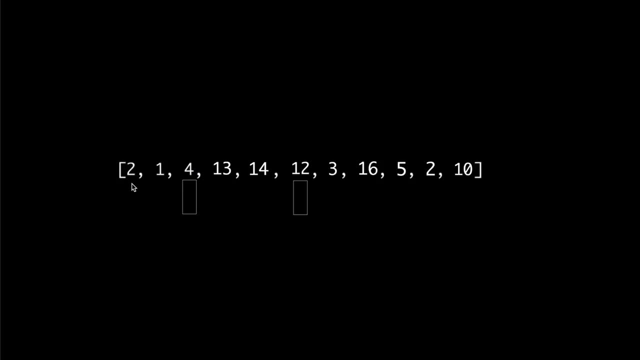 implemented. But before I show you some code, I'm going to give you an overview of how it works, And for that I'm going to use an example where we have an array of 11 elements, just like this one, And to explain it actually I'm going to jump into 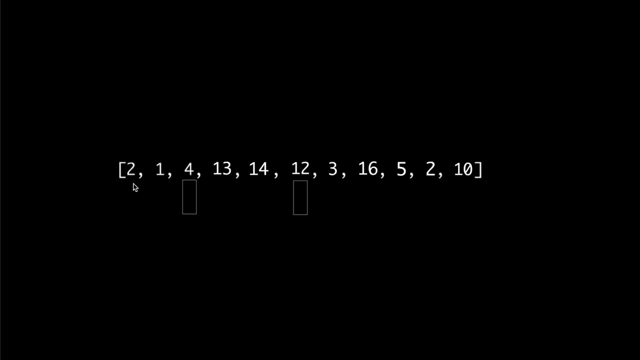 the middle of running this algorithm instead of at the beginning, And I'm doing it that way because I think the middle part is easier to understand, And then I'm going to explain the beginning part later. Anyway, let's say here that we're trying to partition. 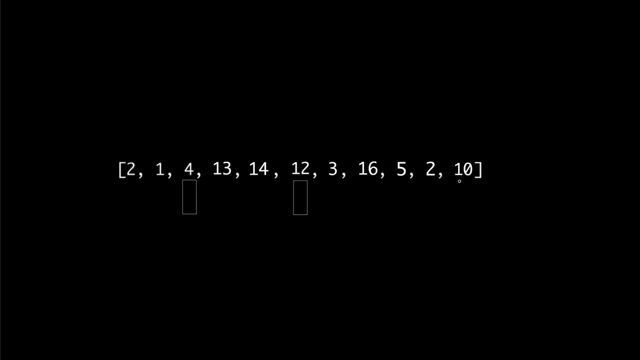 the entire array and our pivot is the last element, 10, right here, And to run this algorithm, we're going to use two indexes: j and i. j will keep track of the current number that we're examining And this is going to be part of a for loop. 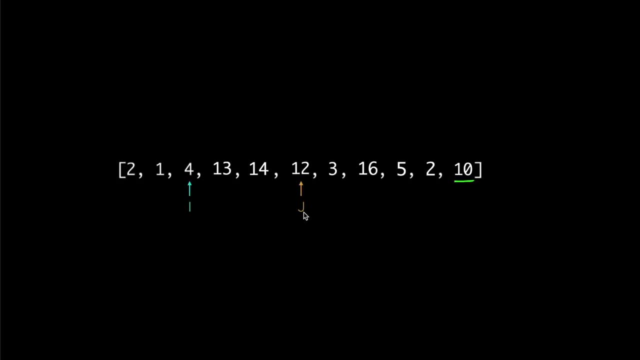 that we're going to use, So that for loop is going to say: move j from the beginning of this array up to the number that's right before the pivots, And currently we're examining this number. let's say, And in each iteration of the for loop, 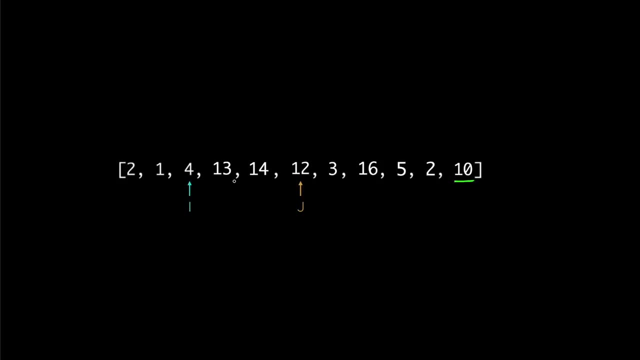 we want to make sure that all the numbers we've seen so far are separated into two groups. The first group is the numbers that are less than the pivots, And the second group is the numbers that are greater than or equal to the pivots. 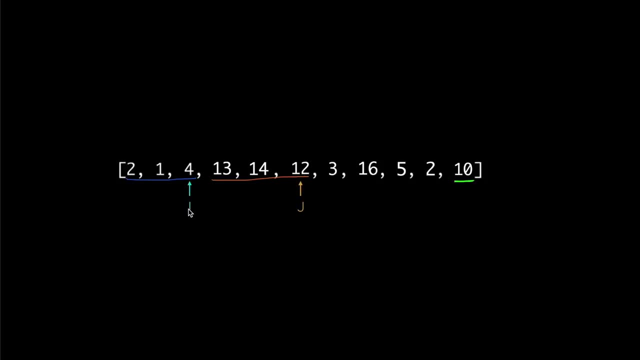 And we want to do it in a way that i this index right here, will always point to the last number out of the numbers less than the pivots. In other words, there are two conditions that we want to always satisfy. The first one is that all the numbers 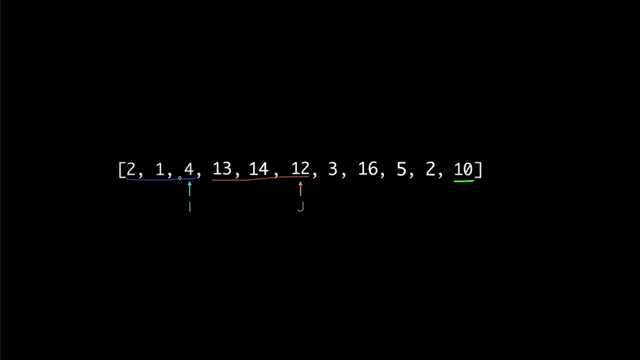 from the beginning up to i are less than the pivots. And the second one is that all the numbers between i and j, not including i, are greater than or equal to the pivots And, like I said earlier, we're currently examining this number 12.. 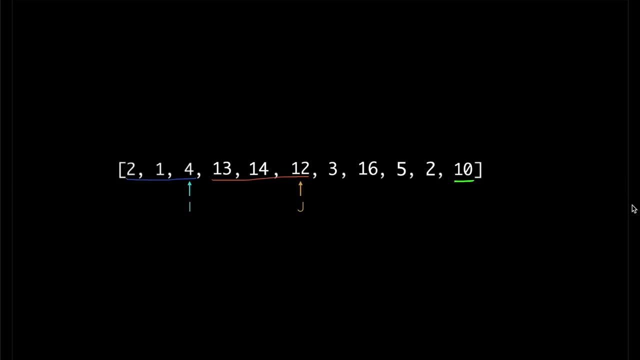 And those two conditions are already satisfied because 12 is already greater than the pivots. So we can move to the next number by incrementing j by 1.. And at this point one of those conditions is not satisfied anymore And we can fix that by doing this. 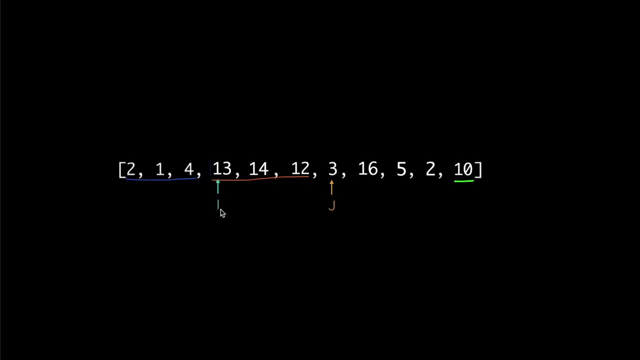 We're going to increment i by 1, or move i over here and then swap the values at i and j, just like that, And that way those two conditions are satisfied again. So all the numbers up to i are less than the pivots. 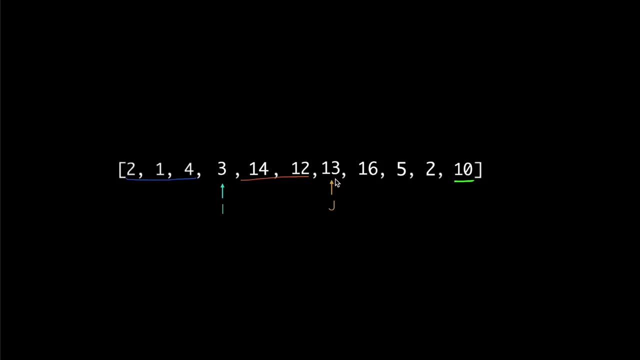 And all the numbers after that, up to j, are greater than or equal to the pivots. So we can keep going, Move j over here, And since this number- 16, is already greater than the pivots, there's nothing to do. 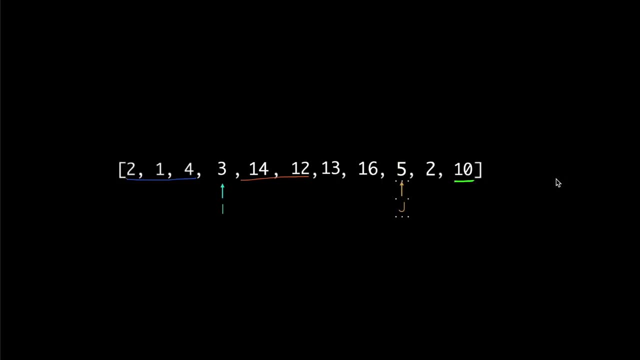 So let's move j over here And, as you can see, the number at j is less than the pivots. so we'll need to do the same thing: Increment i by 1, or move i over here and then swap the values at i and j. 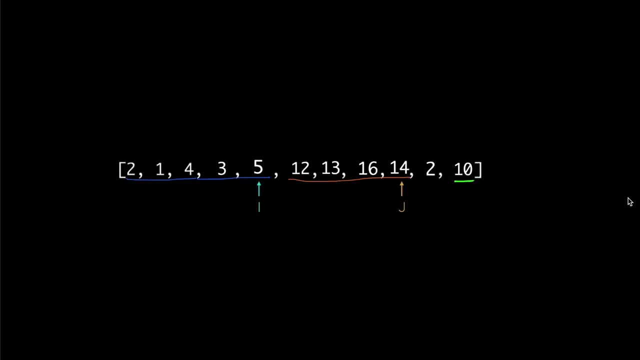 just like that. Okay, let's finish this up by moving j over here, or by incrementing j by 1, and then, doing the same thing, Increment i by 1, and then swap the values at i and j. Alright, and as you can see, 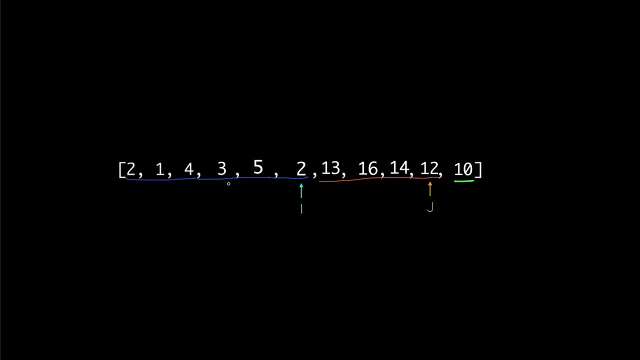 at this point, this array has been grouped into two groups of numbers: the numbers less than the pivots and the numbers greater than the pivots. But the last thing we need to do is we need to make sure that the pivot is between those two groups. 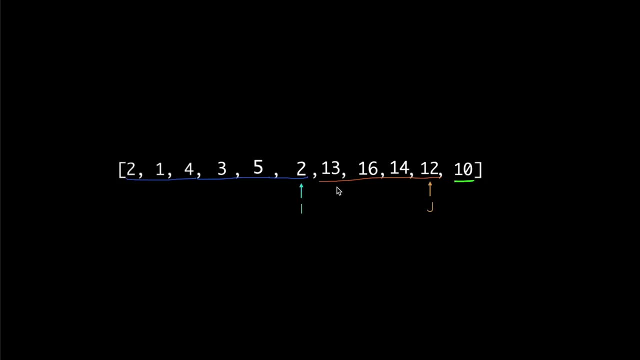 We can do that by swapping the pivots with the value at i plus 1, this value right here. So let's swap those two values, just like that, And then we're done partitioning, Like I said, from our partition function. 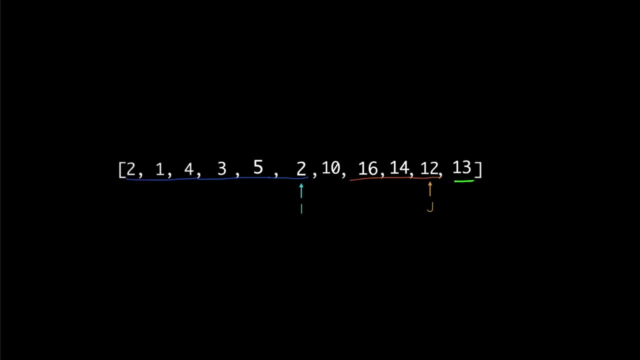 we're supposed to return the index of the pivot, so we can just return i plus 1, because that's the index of the pivot. Okay, so now that we hopefully understand how this partition algorithm works, let's take a look at some pseudocode. 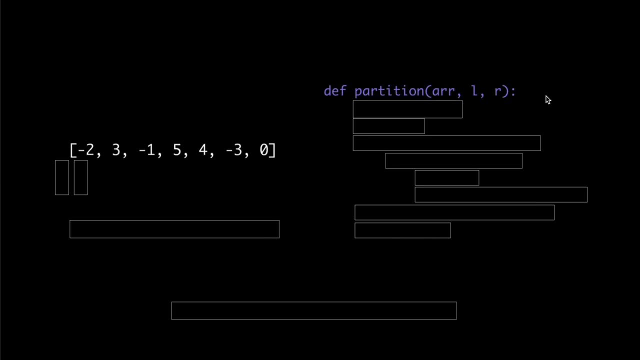 Like I said earlier, we're going to call this function partition and it's going to take three arguments: the given array, l and r, And this function is going to apply partition to the section of the array between l and r. 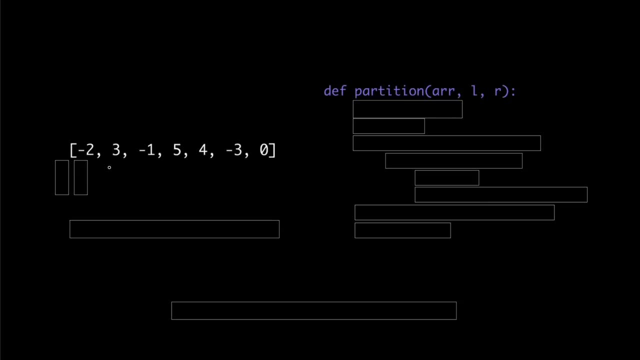 Let's say here, as an example, that we're given this particular array, with l being the beginning of the array, or 0,, and r being the end of the array, or 6 in this particular case, And the first step of this function. 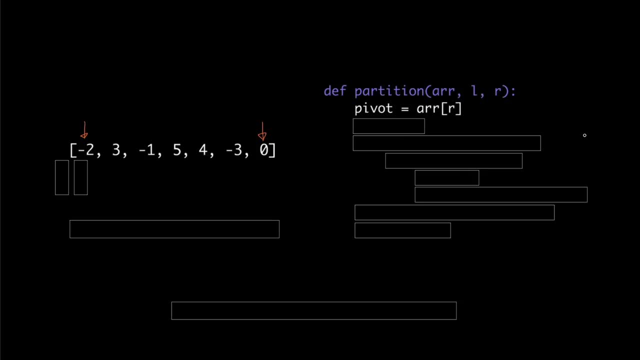 is going to be define the pivot And that's going to be the value at r, or the last element of the section of the array that we are trying to partition, and that's going to be 0 in this particular case. And then we're going to define i to be l minus 1.. 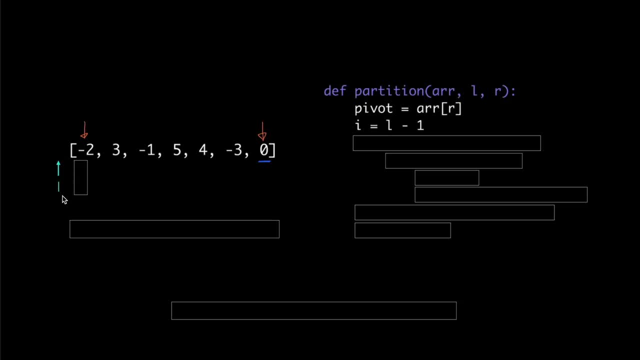 In this particular case, i will be initialized to minus 1.. And then we're going to run a for loop for j, from l, this element up to r minus 1, the last index before the pivot, And in each iteration of this for loop, 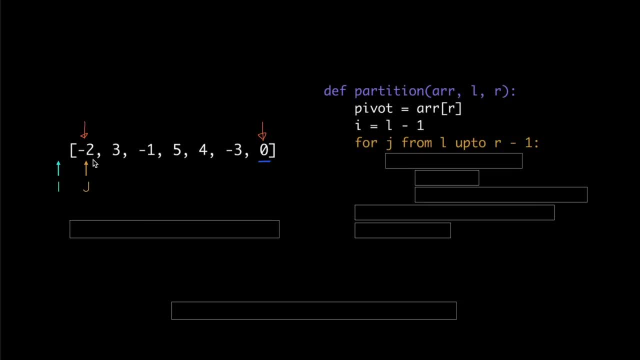 we're going to check if the current number that we're examining, or r of j, is less than the pivot. If that's the case, for example, the current number we're examining, minus 2, is less than the pivot. 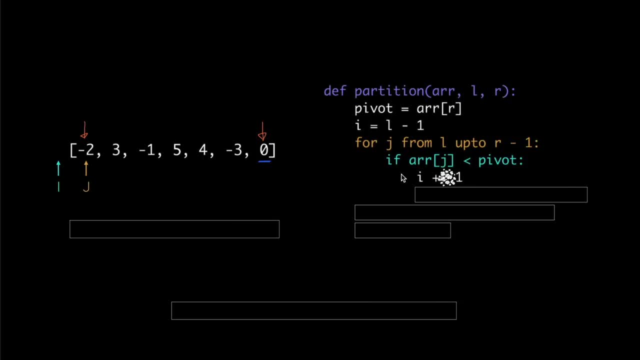 which is 0.. If that's the case, then we're going to increment i by 1.. And then we're going to swap r of i and r of j, So those two numbers happen to be the same number in this particular case. 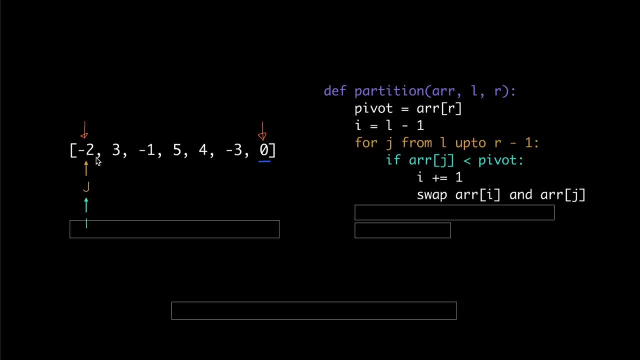 So we're swapping this number by itself and nothing happens. But let's continue with this for loop. So after that we'll move j over here, And since the current number that we're examining- 3, is greater than or equal to pivot. 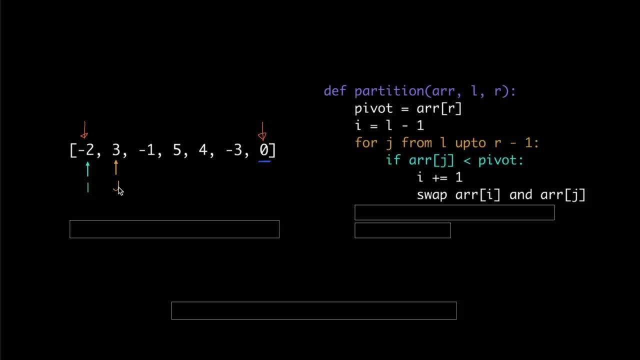 so nothing happens. And so we move j over here, And at that point this number is less than the pivot. so we're going to move i over here, And then we're going to swap the numbers at i and j, And just like that. 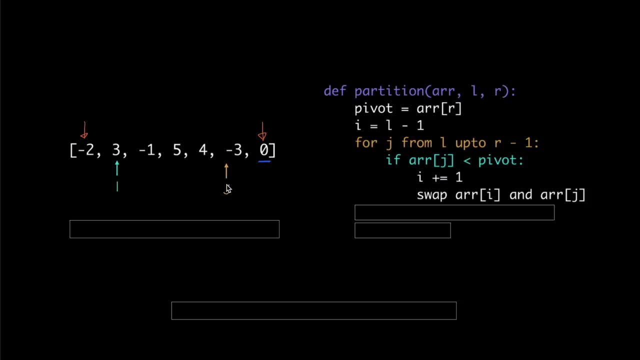 we can keep going with this for loop until j is right here. At that point, our array is going to look like this: j is going to be right here and i is going to be here, Right here. After that, we want the pivot to be. 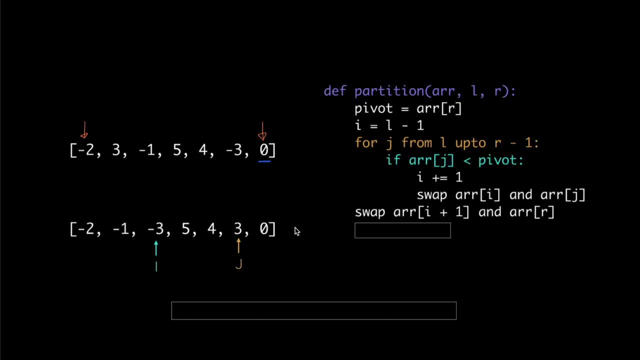 between those two groups of numbers And we can do that by swapping r of i plus 1,. this number right here, 5, and our pivot, r of r. So that's this number and this number, And once it's swapped, 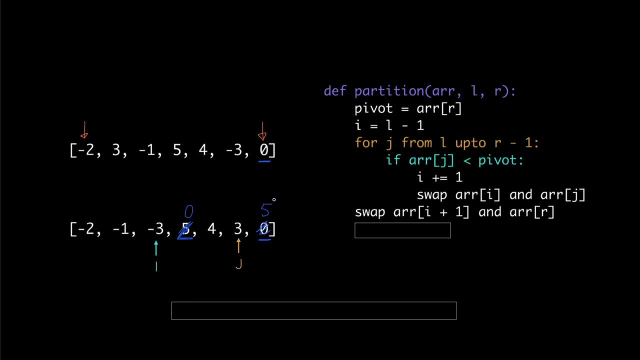 0 will come here and 5 will come here. We just need to return i plus 1, the index of the pivots. OK, so that's my suit code, But you can check my actual implementation in Python and Java at this URL too. 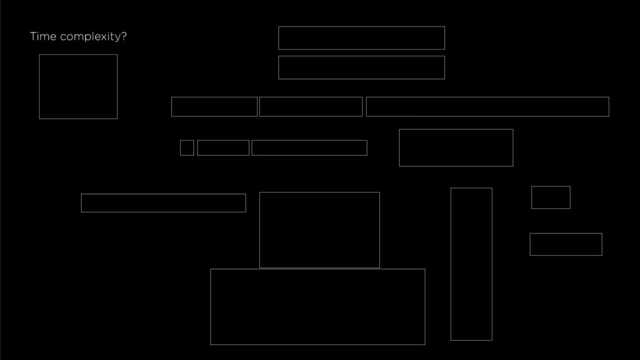 OK, so that's the quicksort algorithm, But what about the time complexity? To understand this, we'll need to consider the best case, the worst case as well as the average case. So let's start with the worst case, That's when the given array 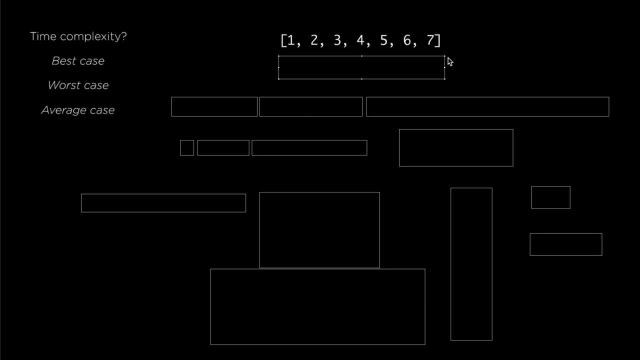 is already sorted, like this one, or when we have a lot of duplicates in the given array, like this one, And actually the time complexity of these two cases will be the same. So let's just consider a case where the given array is already sorted. 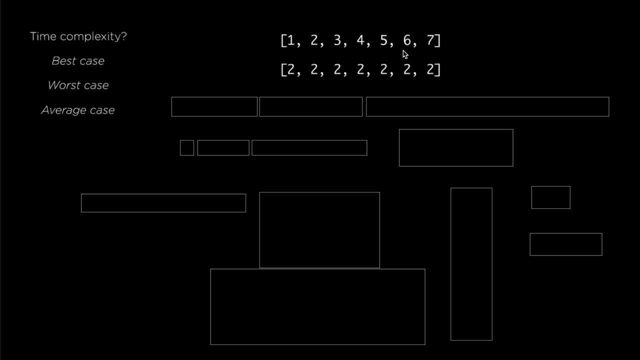 For this particular example, to sort this array with the qs function that we saw earlier, we would call it with the given array: 0 and 6.. So 0, would be right here, the beginning of the array, and 6 would be the index. 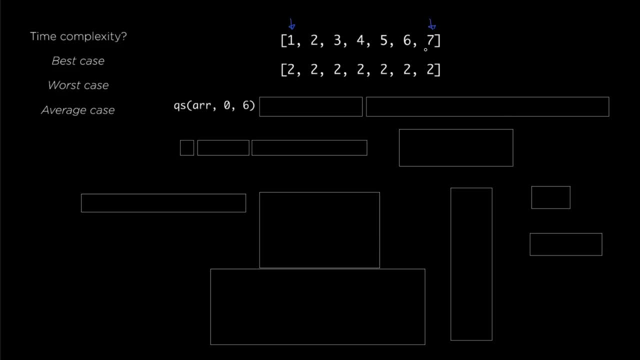 of the last element of the array, And the pivot will be this one, And after running the partition function for the entire array, actually what's going to happen is the pivot will stay here and all the elements will stay where they are, So nothing is going to happen to this array. 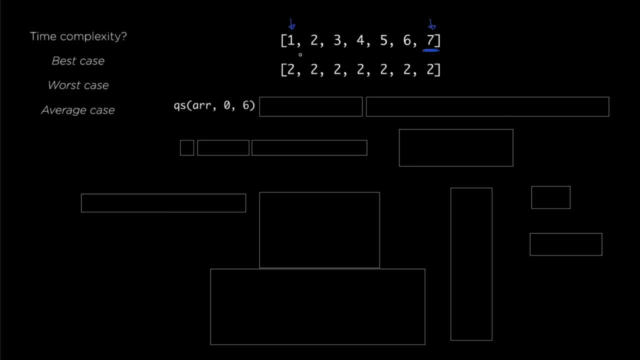 And after finishing partition we'll need to call qs for the rest of the array other than the pivots. We can do that with qs of r and 0 and 5. And we end up doing the same sort of thing over and over again. 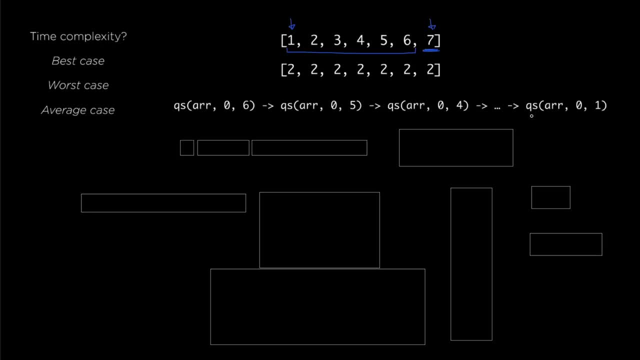 So we would call qs of r and 0 and 4 after that and so on until we get down to qs of r, 0 and 1.. So the pattern we see here is that the number of elements that we need to examine in the qs function. 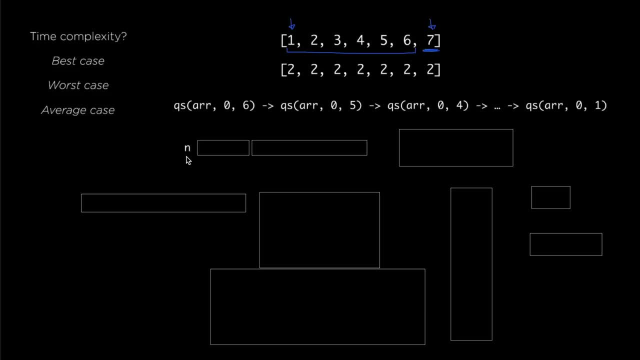 starts at, let's say, n, the number of elements in the entire array, And then we get down to n-1, and so on, n-2, up until 1.. So, as I said, this is the number of elements. 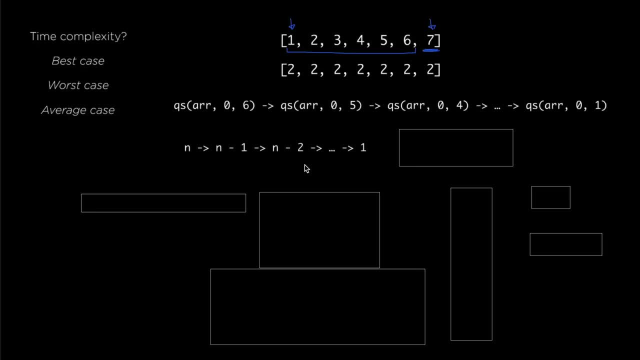 that we need to examine in the qs function each of these numbers, but it's also the number of iterations that we need to go through in our main for loop. To be precise, you might say if we have n elements given to the qs function. 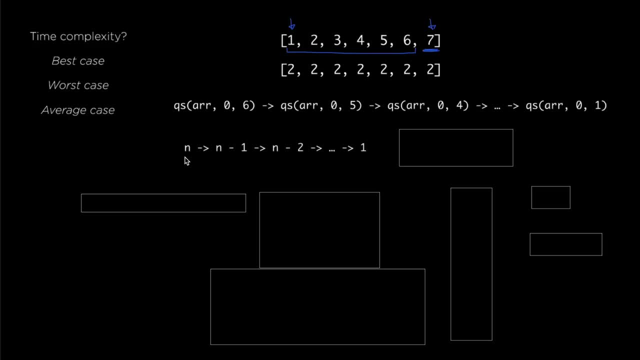 we'll need to go through n-1 for loops in our partition function, but it's roughly n. So if you want to add up the total number of for loop iterations that we need to go through for this entire execution of the function, then we can just add these numbers up. 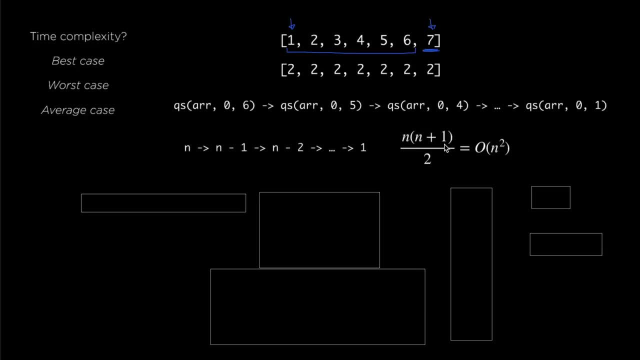 So we get this one n times n plus 1 divided by 2, which is O of n-squared. And that's why we get O of n-squared as the time complexity of the worst case scenario. And what about the best case? 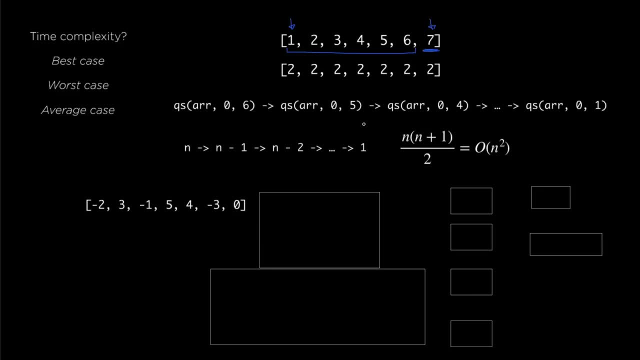 Well, the best case is, every time we chose our pivot, it happens to be the best choice. So it means it happens to be the median, or the closest number to the median, of the given section, of the given array. So, as you can see, in this particular case, 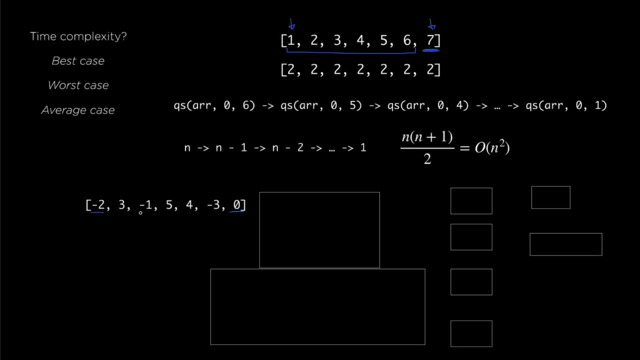 the number of integers less than the pivot is equivalent to the number of integers greater than the pivot. In the best case scenario like that, we would start with n elements that we need to deal with in our qs function and then in the subsequent calls of qs. 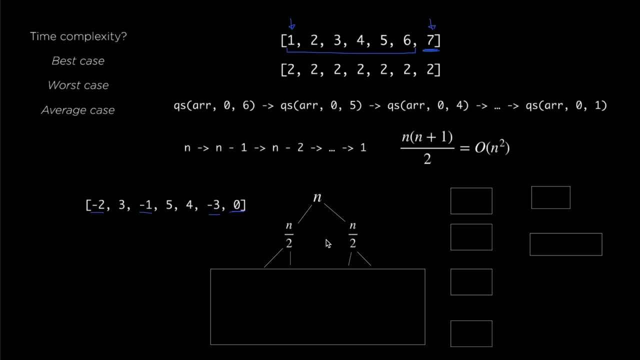 we would have to deal with n over 2 elements in one of the calls and n over 2 in the other one. It's going to be slightly less than n over 2, but it's going to be about n over 2.. 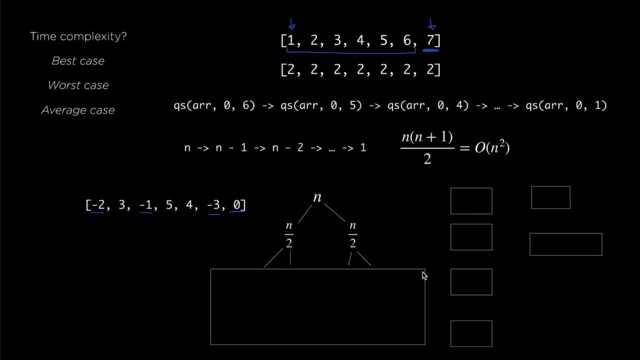 And in the subsequent calls after that we would need to deal with n over 4 elements, and so on until we get down to single elements. And what's interesting here is if you look at each level, if you look at the top level, for example, 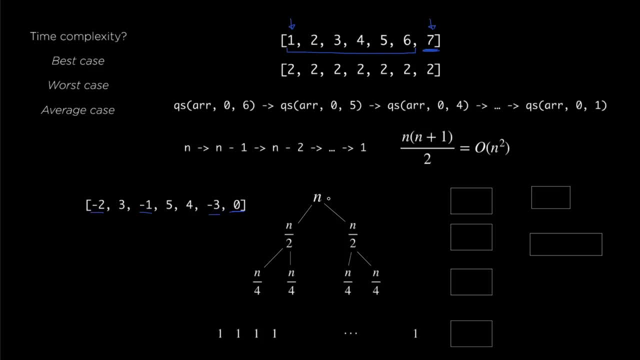 you can see that we would go through about n for loops in our partition function in this level And if you look at the second level we can do the same kind of analysis For this call in the partition function we would need to deal with. 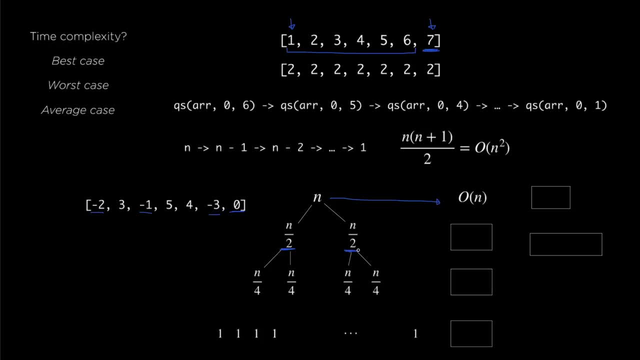 n over 2 for loops, and for this one we'd need to deal with n over 2 for loops as well. So the total number of loops that we need to go through for the second level is going to be of n as well. 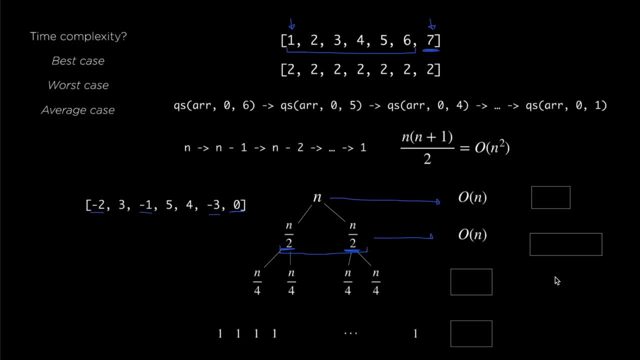 or about n loops. It's going to be the same thing with this level and this level as well, And this kind of analysis will show you that executing everything on each level will take of n in time. And you might say: well, how many levels do we have? 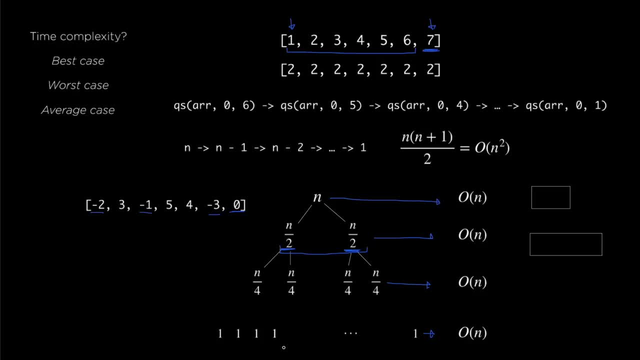 in this recursion tree. Well, we can use the same kind of argument as the one I used in my binary search video to show that the number of levels here is going to be about log n or log 2 of n. So basically what I'm saying here. 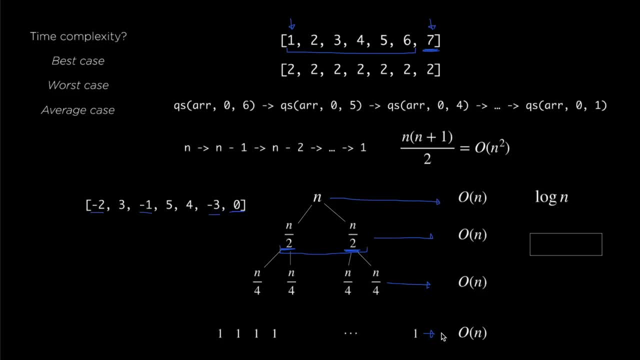 is that we have log n levels here and for each level the time complexity is of n. so to find the total time complexity for the best-case scenario we can just multiply them together and we get of n log n. So that's the time complexity. 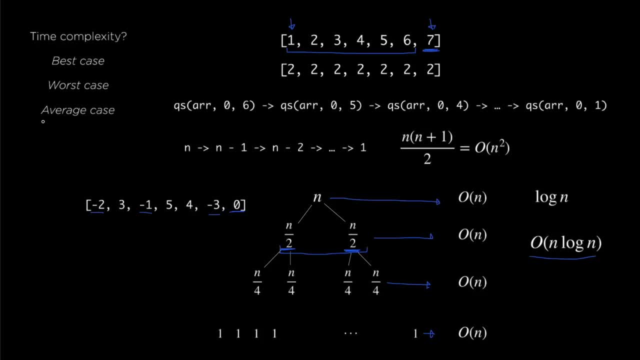 for the best-case scenario. And you might say: what about the average case? Well, it's more tricky to think about, but given a few assumptions, we can actually show that the time complexity for the average case is also of n log n. 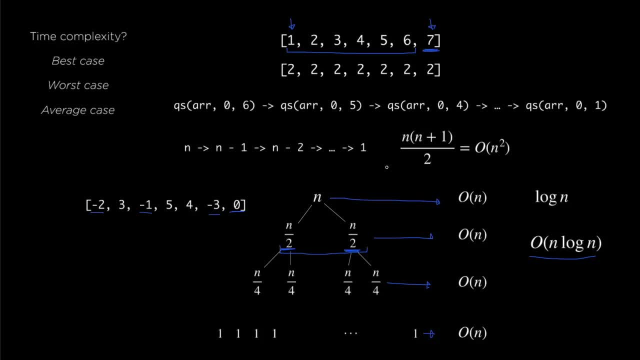 And, by the way, those few assumptions are, first, that there are no duplicates, so we don't have a case like this, and, second, that the ordering of the array is random, And I saw this proof in a book I used as a reference. 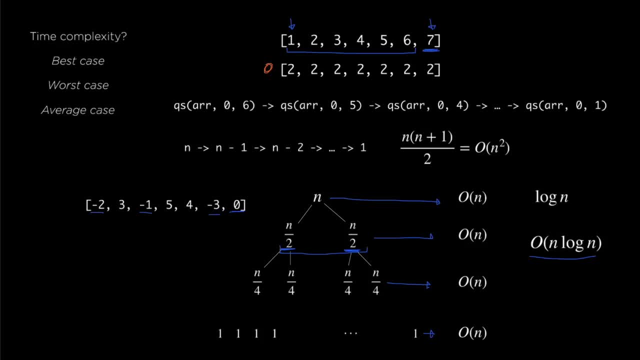 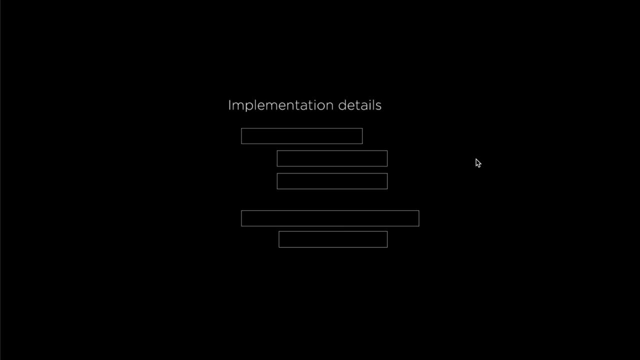 to make this video. so in case you're curious about the proof, I'll put a link to the book in the description below as well. Okay, and before I go, I wanted to mention a few things to note about the implementation details. 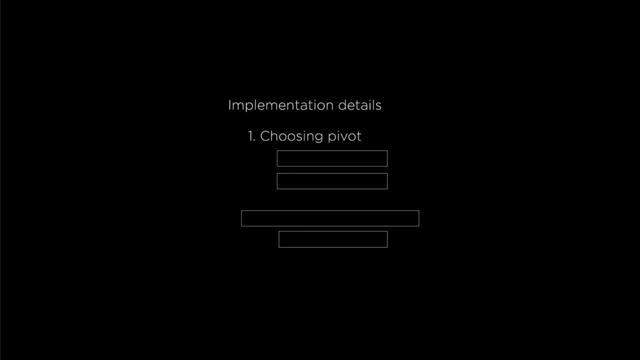 The first one is how to choose the pivots. Of course, in our implementation we chose the last element, but another method is to pick a random element as your pivot Or, equivalently, you can before running our quicksort function. 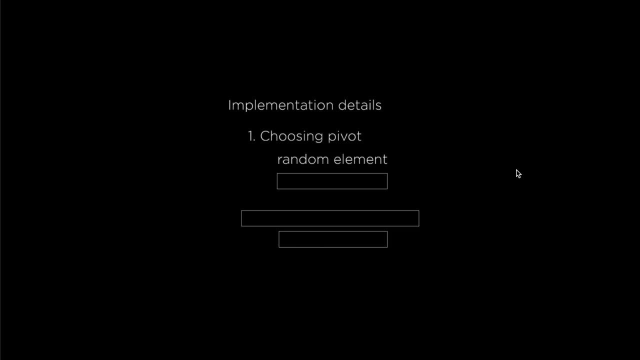 you can reshuffle the given array randomly and then pick the last element as the pivot. And another method for choosing the pivot is called median of three. The idea of this approach is, instead of picking one element, you would choose three elements randomly from the given section. 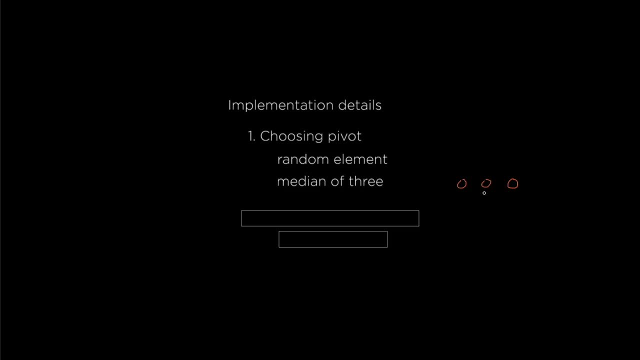 of the given array and then you would pick the median of those three numbers And that way you'll be able to decrease the probability that you would pick a bad pivot for the given section of the given array. Okay, and the second thing. 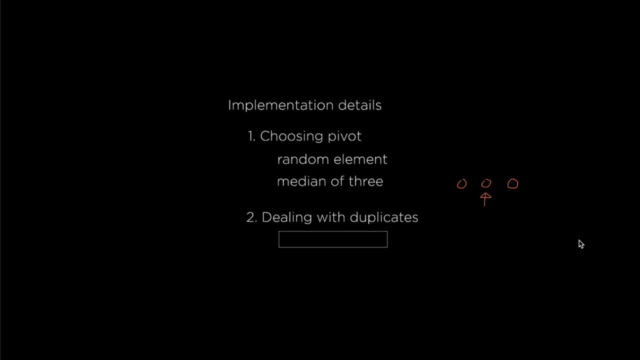 I wanted to discuss is dealing with duplicates Because, as we saw, quicksort doesn't perform well when there are a lot of duplicates in the given array. One way to deal with this is called three-way quicksort, In case you're curious about it. 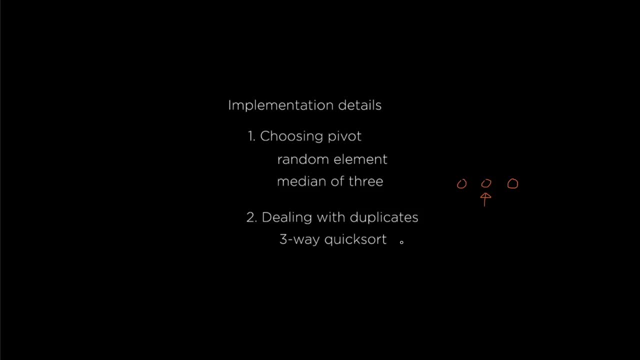 I'm going to put a link to a page that describes this method, But the idea of this method is that, instead of dividing the given section of the given array into two groups, we divide it into three groups. The first group is going to be: 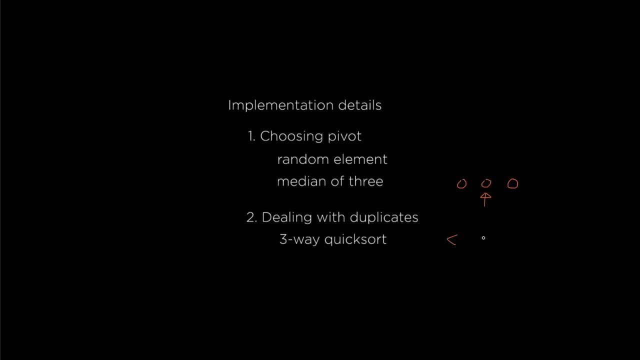 the numbers less than the pivots. The second group is going to be the numbers equal to the pivots And the third group is going to be the numbers greater than the pivots. Again, in case you're curious about it, I'm going to put a link to a page.